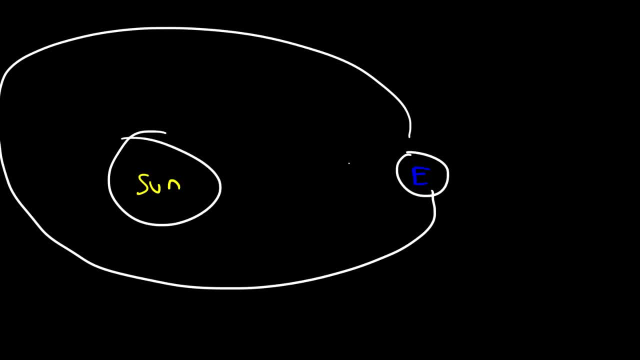 motion in this example. so what keeps the earth in orbit around the Sun? in this case it's a gravity, and gravity provides the centripetal force. gravity pulls the earth towards the Sun, but the earth wants to fly outward, towards outer space, so instead it turns. so gravity keeps the earth in orbit around the Sun. so, as you, 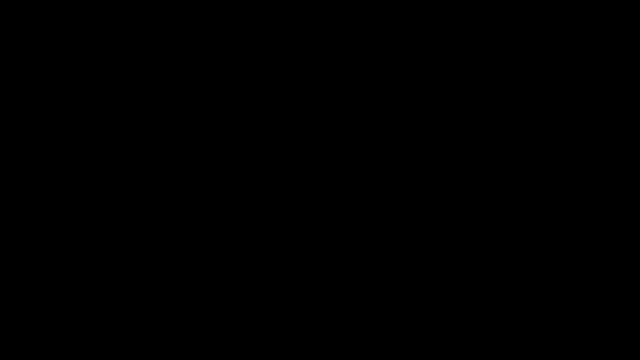 can see, the centripetal force is not really a new kind of force. it's a force that's provided by another kind of force. so any force you can see- the centripetal force is not really a new kind of force, it's a force that causes an object to move in a circle- can be labeled as a centripetal. 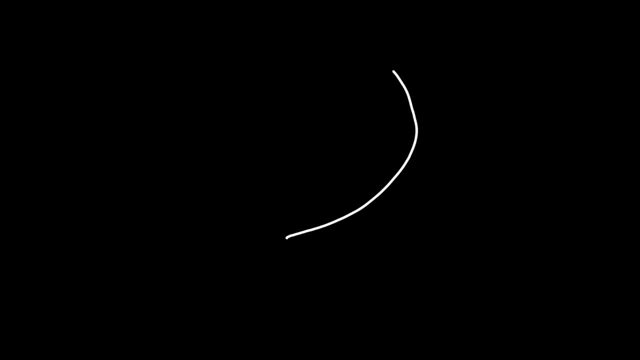 force. so another example is, let's say, if you have a car turning, in this case the static frictional force provides the centripetal force. it allows the car to make that turn on a road. another example that you won't see in this video, but you'll learn more about it in the next semester of physics is the magnetic. 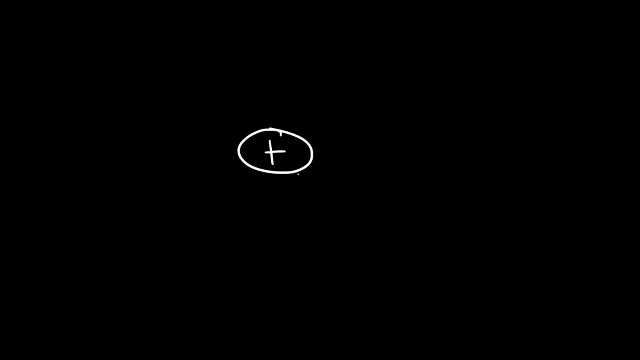 force. let's say if you have a proton or any positive charge and this positive charge is moving towards the right and a magnetic field. let's say it's. going into the page in physics 2 you'll see it's represented by an X symbol. a dot means. 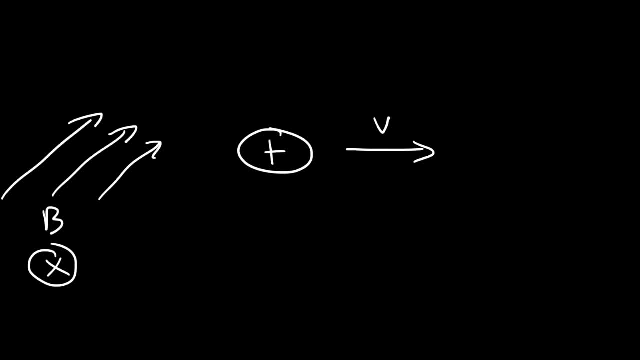 out of the page. so the magnetic field is going into the page and this charge is moving towards the right, it's going to field a magnetic field. I mean a magnetic force that's going to cause the proton or the positive charge to turn. and so whenever you have a moving charge in a magnetic field, that 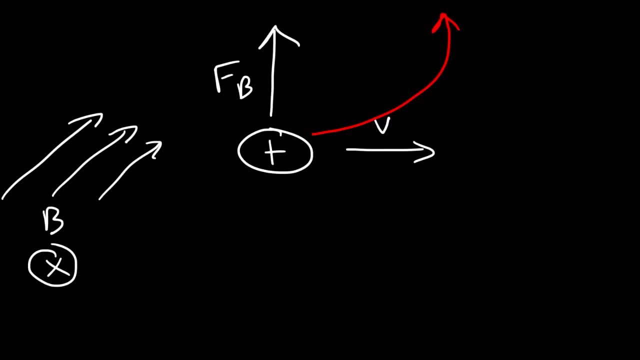 charge is going to turn, it feels a magnetic force exerted on it by the magnetic field, and so this magnetic force can behave as a centripetal force because it's causing the object to turn. so those are the main four examples that you'll see in physics in the case of a 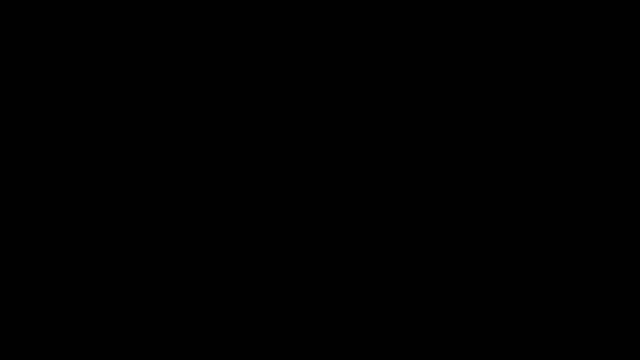 rope, tension can provide the centripetal force. if an object is moving the circle- in the case of planets, it's gravity. in the case of a car turn, it's static friction, and if you have a moving charge in a magnetic field, it's going to be the 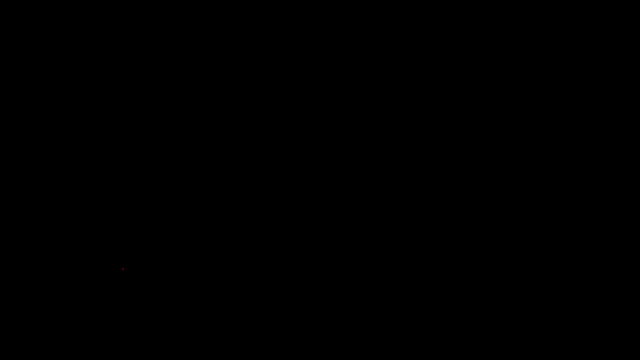 magnetic force that provides the centripetal force. so how can we find the equation of the centripetal force now? according to Newton's second law, the net force is equal to the mass times acceleration. so the centripetal force is mass times the centripetal acceleration. 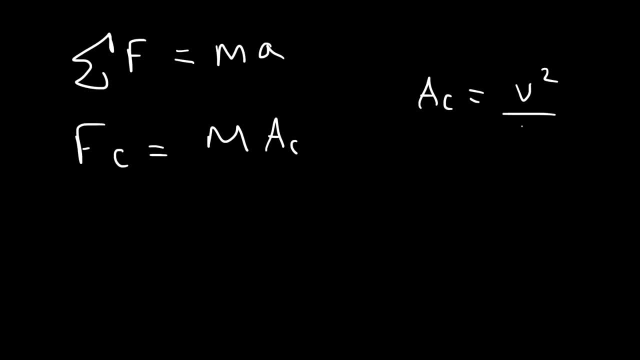 and the centripetal acceleration is v squared over r. so the centripetal force is m, v squared over r. it's directly proportional to the mass and it's proportional to the square of the speed, and it's inversely related to the radius of the force. 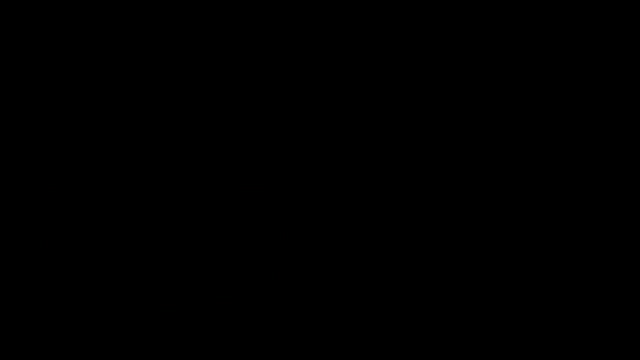 of the circle. now there are some other things that you need to know about this equation. for instance, whenever the mass increases, you need to know that the centripetal force will increase as well. if the speed increases, the centripetal force will increase, and if you increase the radius of the circle, the centripetal 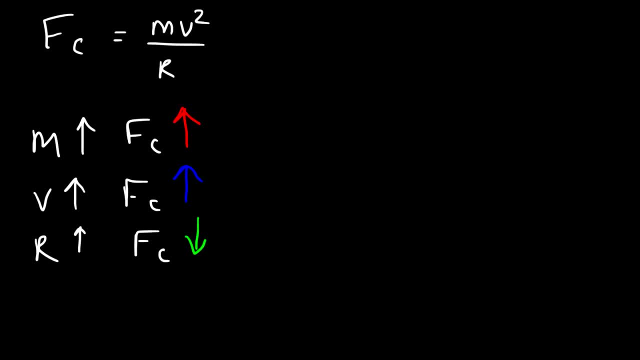 force will decrease. so imagine if you're driving a car and if you make a sharp turn. if you make a sharp turn, you're going to experience a very large centripetal force. you're going to feel like you're flying out of the window. if you decrease the radius, the centripetal 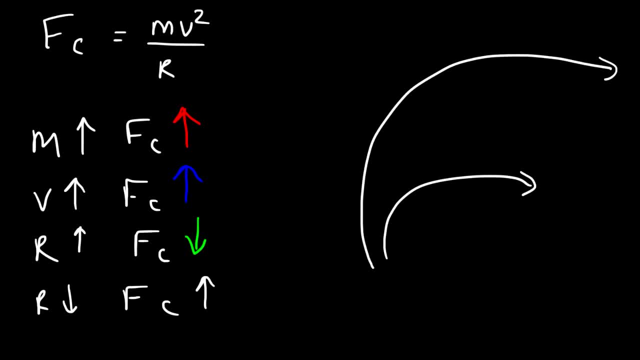 force will increase. but if you make a wider turn, you won't feel like you're flying out of the window as much, because the centripetal force is a lot less. if you increase the radius of curvature now, if you try to make a wide turn at a very high speed, you're going to feel a much larger centripetal force and 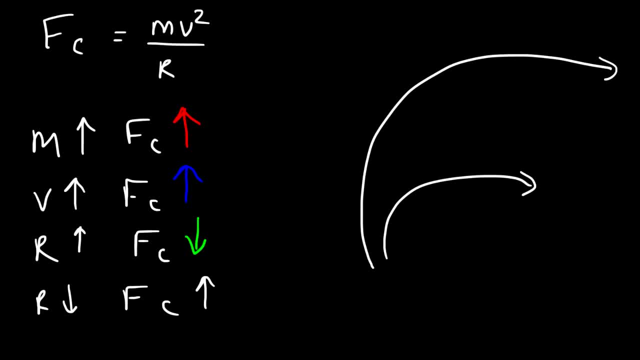 if you make a sharp turn with a very high speed, you might actually fly out the window. so that feeling that you get when you make a turn, you can increase or decrease it. so if you want to decrease that feeling when you're turning, just decrease the speed and increase the turn, the radius of the turn, and you won't. 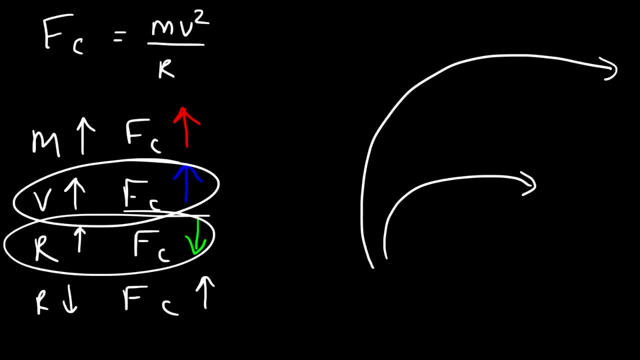 feel that centripetal force effect, as you would when you make a turn. so just make a wider turn at a slower speed. now, if you want to fly out the window, drive fast and make a sharp turn. i would not recommend that, though. now here's a. 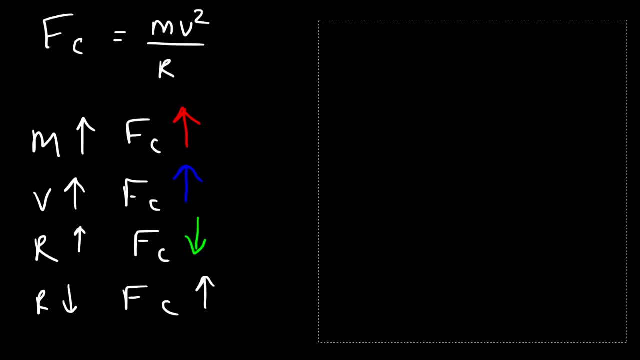 question for you: if you double the mass, what effect will that have on the centripetal force? if you double the mass, the centripetal force will double it. if you triple the mass, the centripetal force will triple. to answer questions like that, just plug it in into the formula. everything else that doesn't. 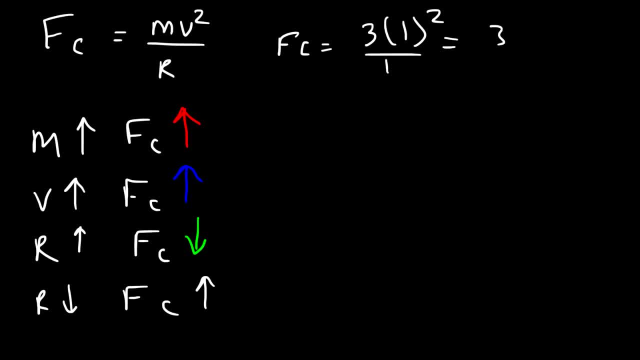 change. replace it with a one, so you get three. likewise, if you double the speed and keep everything constant, the centripetal force will increase by a factor of four. now what if you double the radius of the circle? what's going to happen? the centripetal force will be one-half of its original value. and if you reduce? 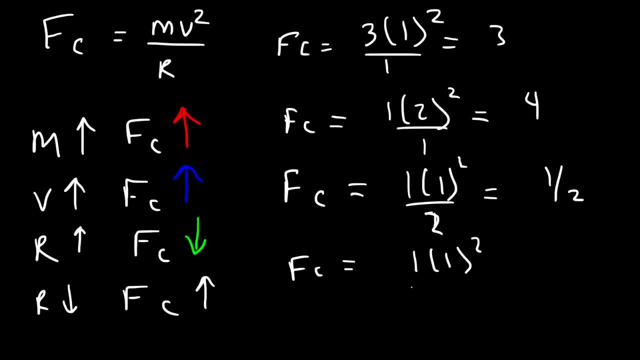 the radius to one-half, the centripetal force will be one over one-half, which is two. it's going to double. now what if you triple the mass, double the speed and decrease the radius by a factor of three? what effect will that have on the centripetal force? so if you triple the 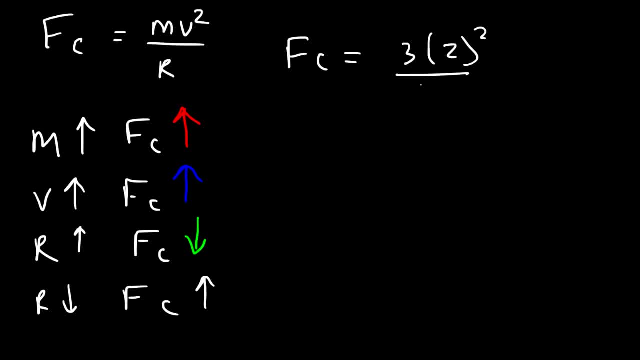 mass, double the speed and reduce the radius to one-third of its value. two squared is four, and three times four is 12. 12 divided by one-third is the same as 12 times 3, so it's 36. the centripetal force will increase by a factor of 36. now I'm 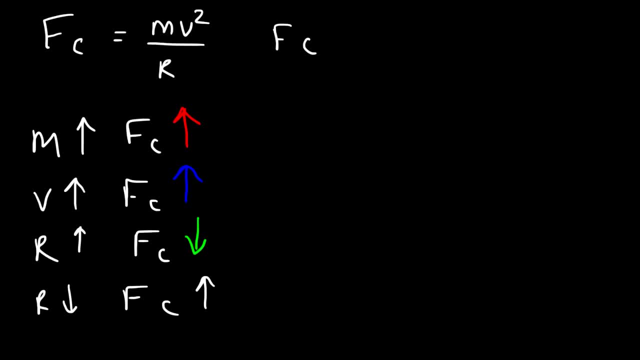 even another example. let's say, if you quadruple the mass, triple the speed and reduce the radius to one-third of its value, go ahead and find the effect that it will have on the centripetal force. so we quadruple the mass, triple the speed and the radius is one-fourth, so it's four. 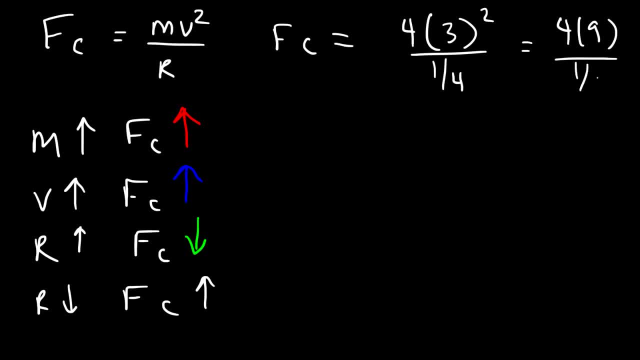 times 3 squared: 3 squared is 9, and 4 divided by one-fourth that's like four times 4, that's 16. so we got 16 times 9. 10 times 9 is 96, times 9 is 54. so this adds up to 144. so if you quadruple the mass, triple the speed and 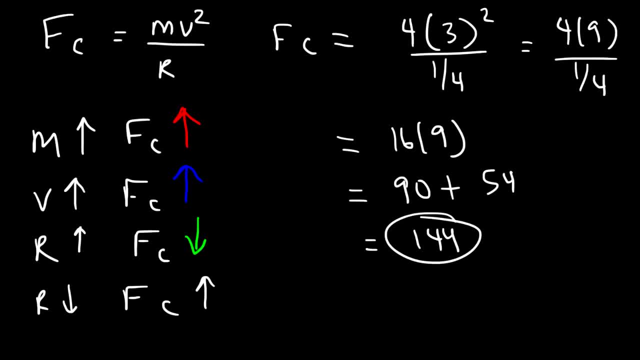 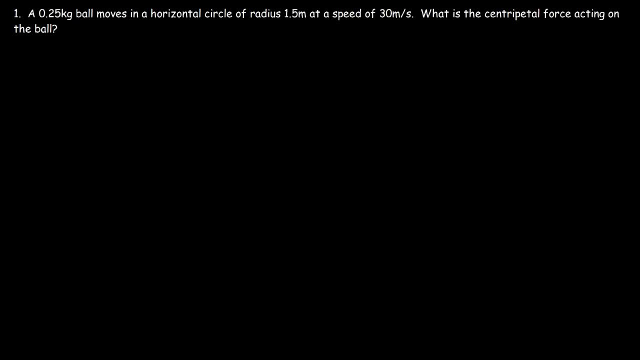 reduce the radius to one-fourth of its value. the centripetal force will be 144 times greater than its current value. now let's move on to some practice problems. a point: 25 kilogram ball moves in the horizontal circle of radius 1.5 meters. 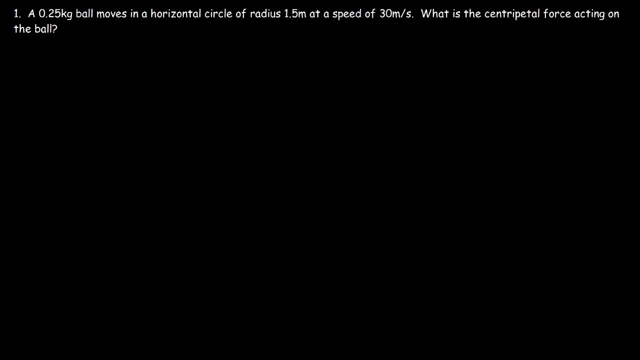 at a speed of 30 meters per second. what is the centripetal force acting on the ball? so here's the ball. it's moving in a circle, the centripetal force is always directed towards the center of the circle and it's equal to m v squared divided by R. so we have everything that. 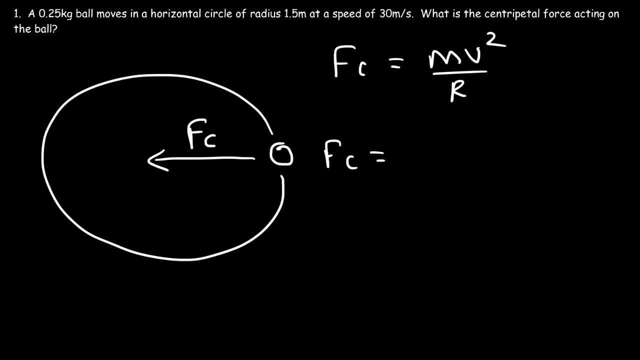 we need. we have the mass of the ball, which is point 25 kilograms, and we have the speed, which is 30 meters per second, and the radius is 1.5. 30 squared is 900 and 900 times point 25 is 225, if you. 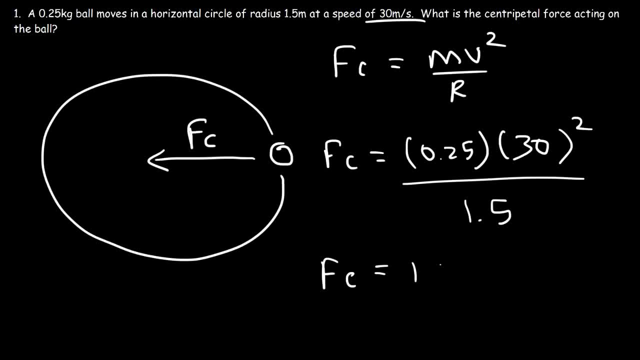 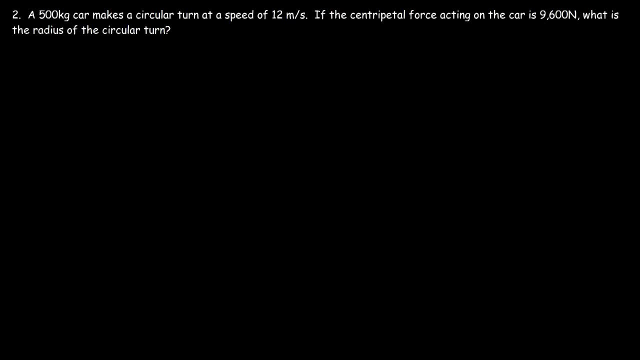 divide that by 1.5, you're gonna get 150. so that's the centripetal force acting on this ball. it's 115 units. now let's move on to this example. a 500 kilogram car makes a circular turn at a speed of 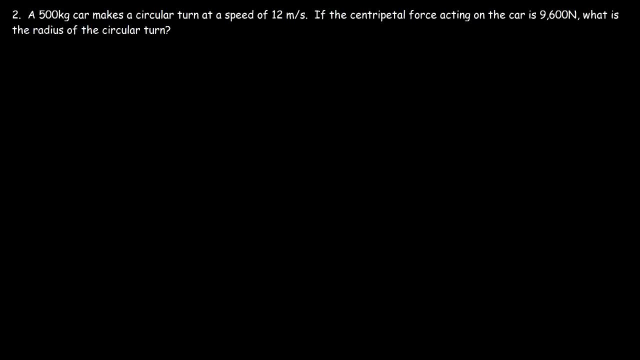 12 meters per second. If the centripetal force acted on the car is 9,600 Newtons, what is the radius of the circular turn? So we have the mass, which is 500 kilograms. we have the speed, which is 12. 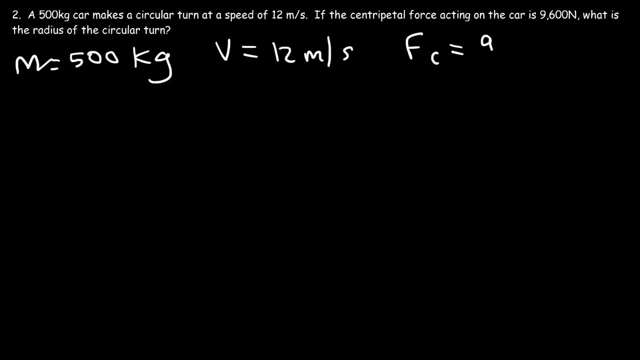 meters per second, and we have the centripetal force, which is 9,600 Newtons. All we need to find is r, the radius. So let's start with this equation and let's rearrange it to get r. So I'm going to multiply both sides by r, and so these: 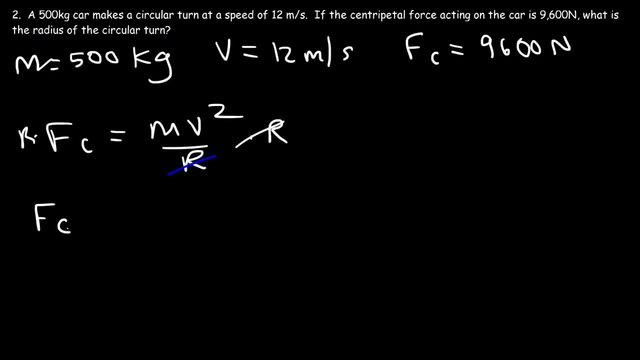 will cancel. So I have the centripetal force times. the radius is equal to mv squared. Next, I'm going to divide both sides by the centripetal force, So the radius of the circle is going to be the mass times, the square of the. 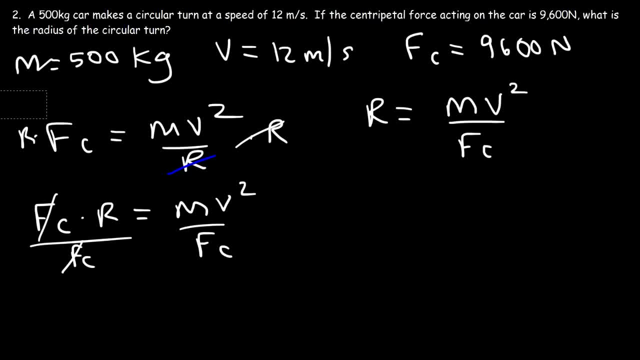 speed divided by this centripetal force. So this is the formula that we need for this problem. So let's go ahead and get the answer. So it's going to be the mass, which is 500 kilograms multiplied by a speed of 12 meters per second squared. 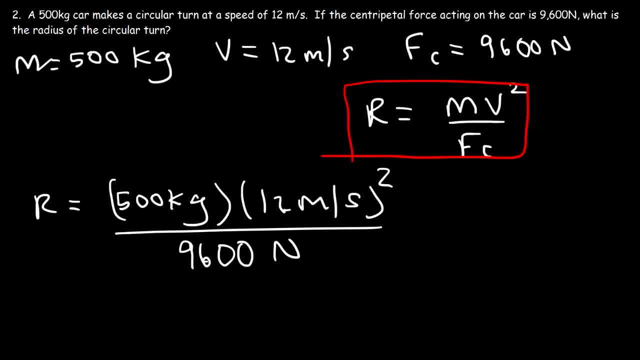 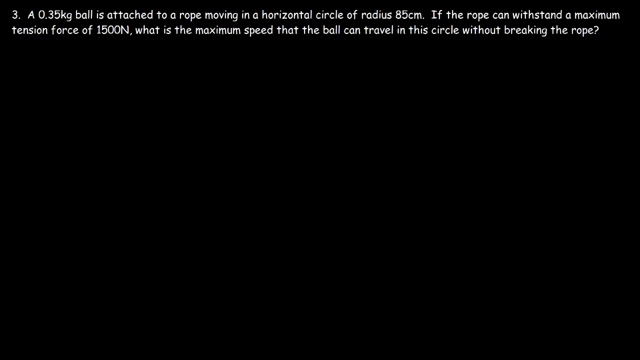 divided by the centripetal force of 9600 Newtons, 12 squared times 500 is 72,000.. And if you divide that by 9600, you're going to get a radius of 7.5 meters. And that's it for this problem. 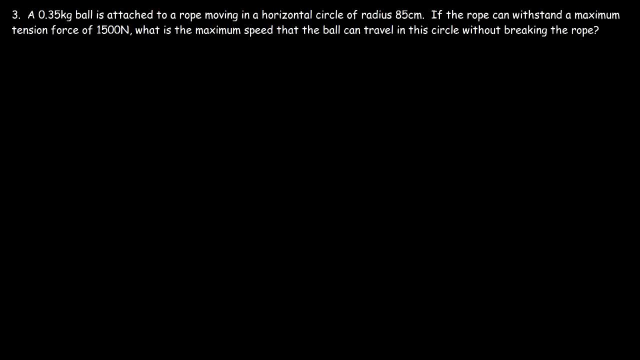 A 0.35 kg ball is attached to a rope moving in a horizontal circle of radius 85 centimeters. If the rope can withstand a maximum tension force of 1500 Newtons, what is the maximum speed that the ball can travel in this circle without breaking the rope? 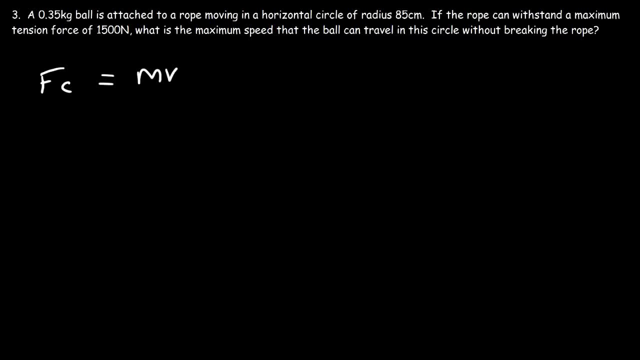 So in this problem we need to calculate V, the maximum speed. So let's solve for V in this formula. So what I'm going to do is I'm going to multiply both sides by r over m. Now the reason why I'm doing that is to cancel the radius on the right side and also to cancel 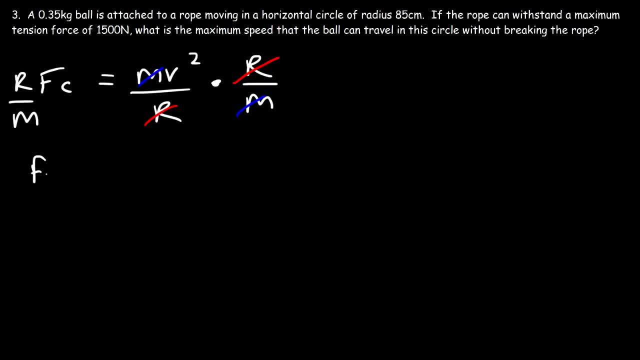 the mass. So all I have left over on the right side of the equation is V. So now I need to take the square root of both sides. So V is equal to 0.35.. V is equal to the radius times the centripetal force divided by the mass. with the square 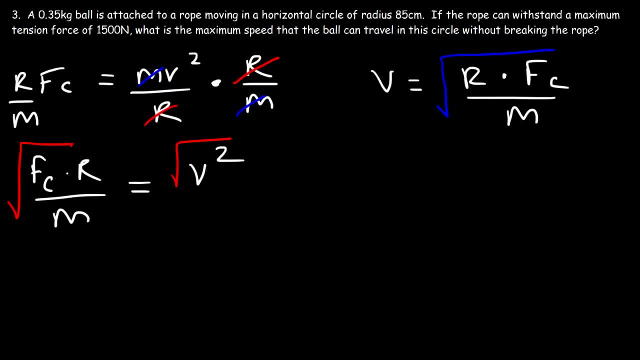 root symbol. So now let's plug in everything that we have into this formula. The radius is 85 centimeters And we need to convert that to meters. One meter is 100 centimeters, So to convert it, take 85 divided by 100 and that will give you 0.85 meters. 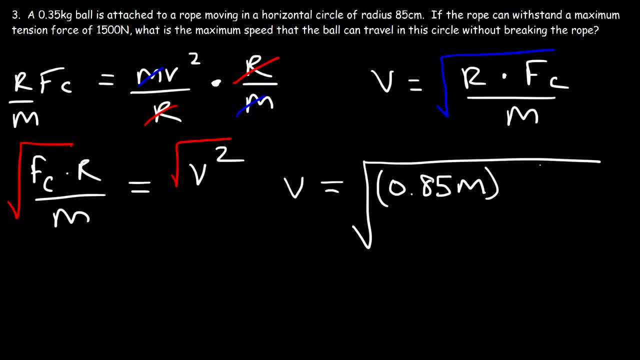 This will give you 0.85 meters. This will give you 0.85 meters. The centripetal force is going to be the maximum tension force, which is 1500 newtons. Whenever you have an object moving in a horizontal circle and if it's attached to a rope, the 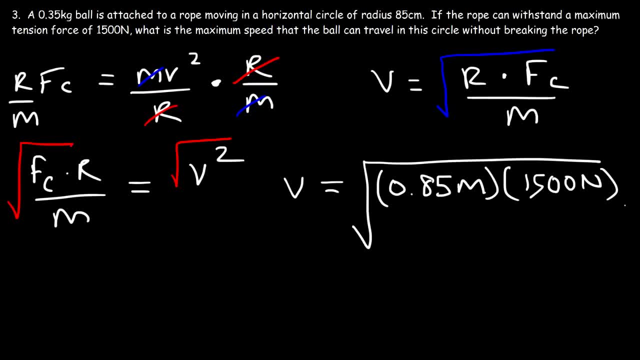 tension force is approximately equal to the centripetal force if the ball is moving fast enough. If not, you're going to have what is known as a tetherball experiment and it's not going to be the same. But if it's moving fast enough, it's going to be the same. 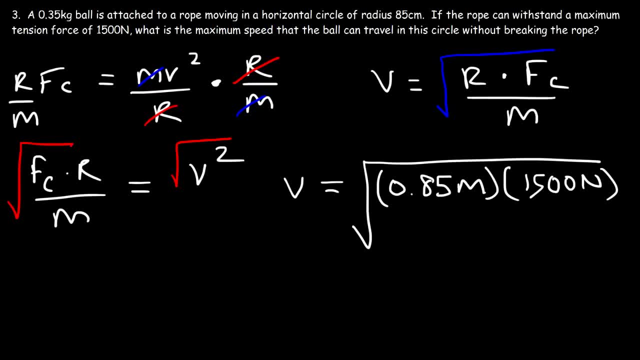 It's going to be the same. You don't have to worry about the weight force of the ball. It's going to be insignificant. But I'm going to go into more detail into that topic in another video. Right now let's plug in the mass, which is 0.35.. 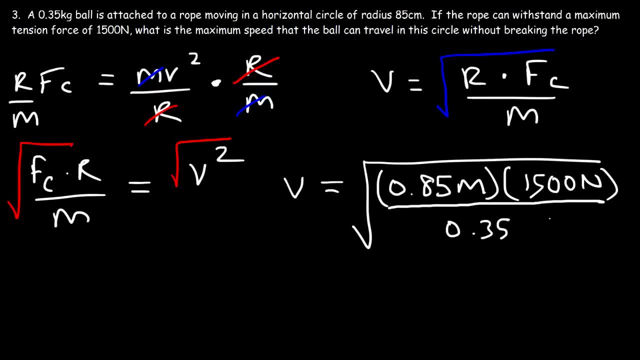 0.85 times 1500, that's 1275.. If you divide that by 0.35, you should get like 3643. if you round it to nearest whole number, take the square root of that number and then the maximum speed is going to be. 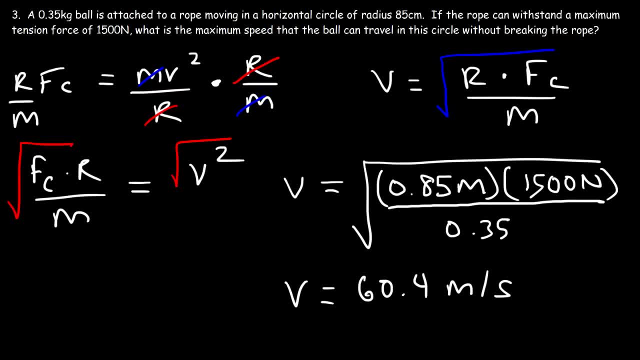 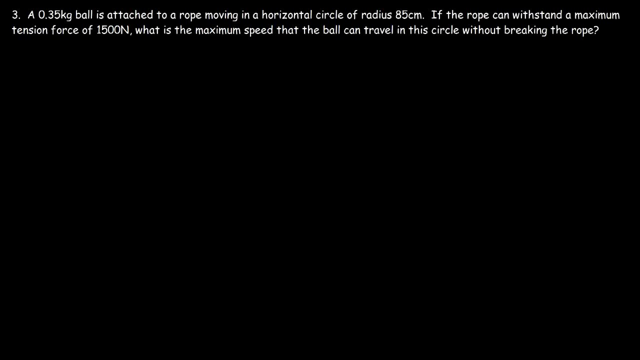 60.4 meters per second. so now you know how to calculate it, if needed. but now let's go over some free body diagrams. now imagine if you're holding a rope in your hand that's attached to a ball and if you spin it fast enough in a 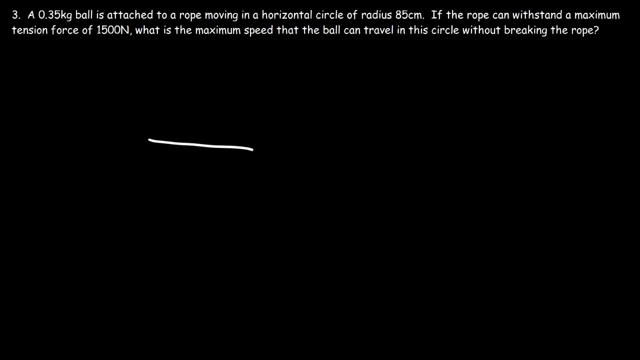 horizontal circle. it's going to look something like this: if it's going fast enough, it's going to appear nearly horizontal. if it's not going fast enough, it might be slightly at an angle, and if it's going slow, the angle is going to be larger. so it's going to look like this. 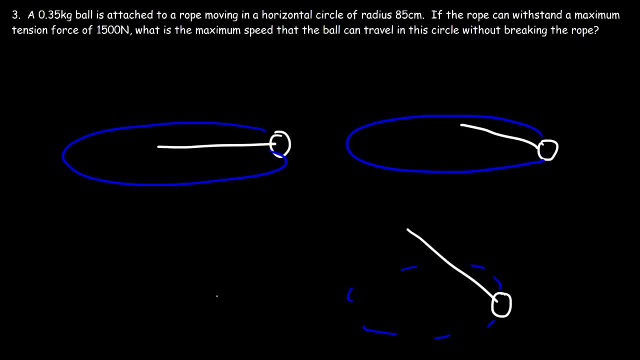 now the tension force is the force in the rope, so that's going to be the tension force. that tension force has an X component and the Y component, which I'm going to call FTX and FTY. now the ball also has a weight force, MG, so this: 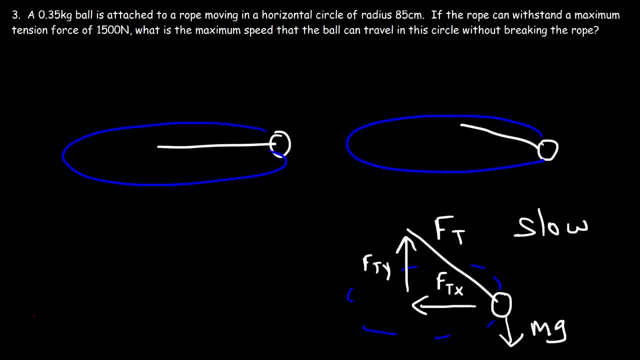 if it's moving relatively slow, this angle is going to be significant. now. the centripetal force is the force that's going to keep it moving in a circle, so it's the horizontal component of the tension force. so when a ball is moving slow, FTX is equal to the centripetal force. this is always true. 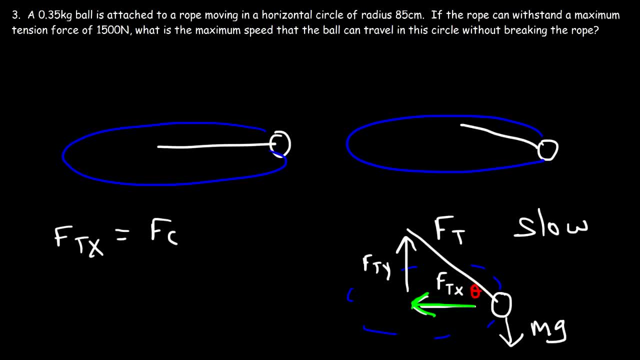 but I'll talk more about when it's moving fast. FT Y is equal to the weight force. this component balances the weight force. now, if you want to find a tension force, it's going to be the square root of FT X squared, plus F, T Y squared. to find FT x, you need to find the centripetal force. 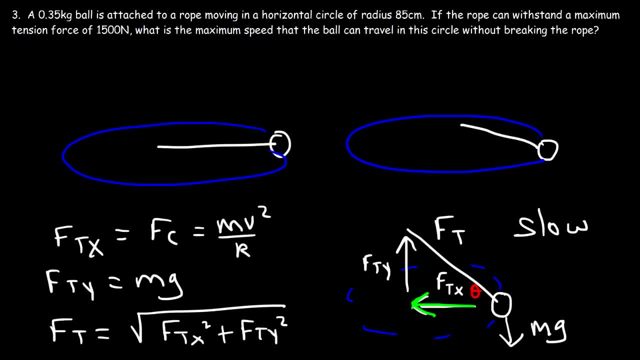 which is MV squared over R, and then FT Y is mg. so if you want to get the exact answer for the tension force, Here's the equation you can use: FTX is MG, right? No, I take that back. FTX is MV squared over R. So you have MV squared over R squared plus FTY squared, which is: 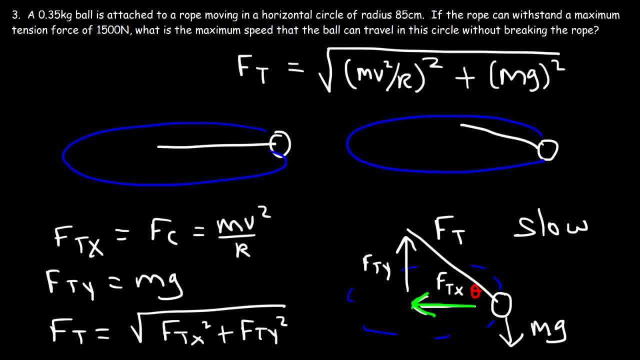 MG squared. So for any situation, this will be the exact answer for the tension force. Now, if the ball is moving fast enough, it's going to look like this: Now we can't really see anything, so I'm going to use this picture. This is still going to be FT and you're still 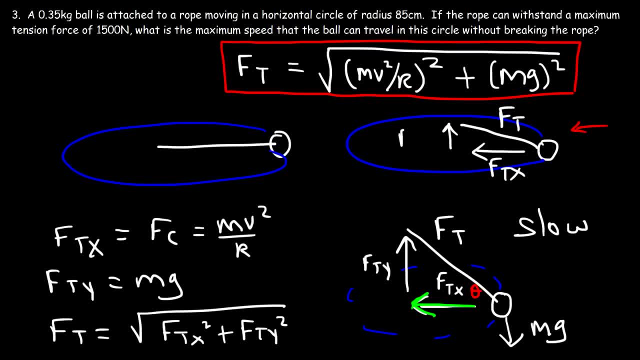 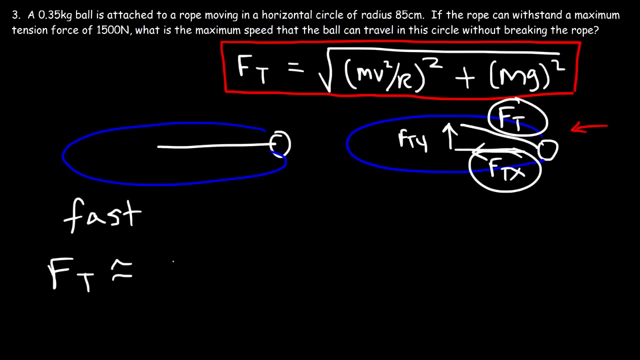 going to have FTX and FTY. But when it's nearly horizontal, FT is approximately equal to FTX. FTY will be negligible. So if the ball is moving fast, you could say that FT is approximately FTX, which is the centripetal force. So that's going to be MV squared over R. 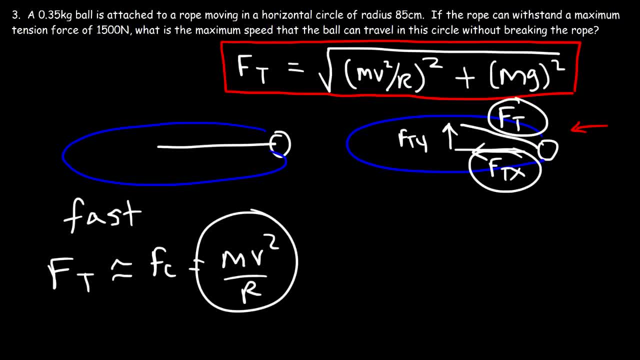 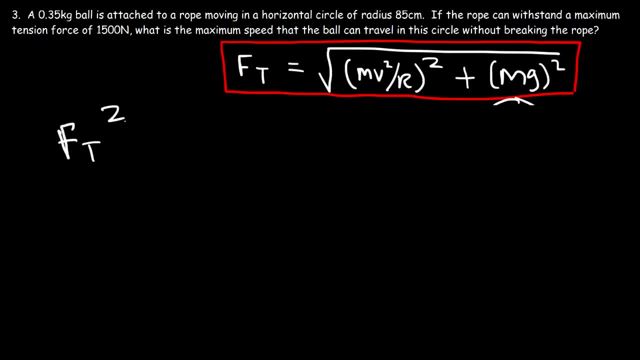 Let's square both sides. So I'm going to have: FT squared is equal to MV squared over R squared plus MG squared. So the tension force is 1500.. The mass is 0.35.. We don't have the value of V. 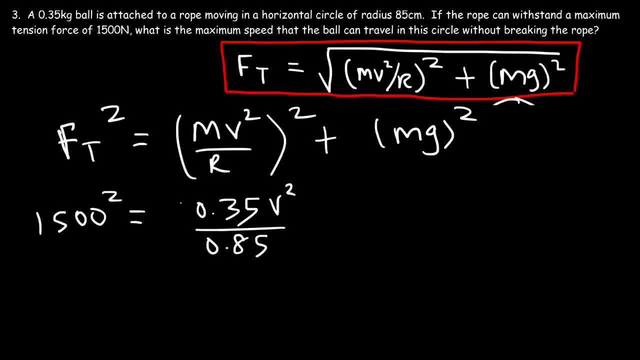 R is going to be 0.85.. And this is squared, And then we have MG squared, So that's 0.35 times 9.8 squared. Now, 1500 squared, that's a big number, That's 2,250,000.. 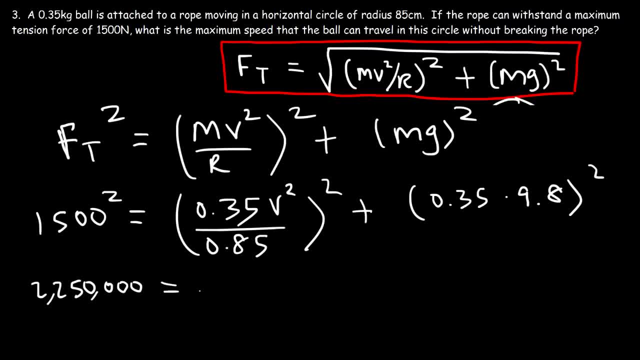 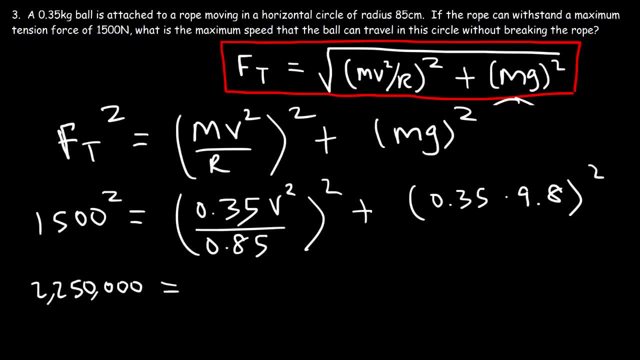 And then it repeats: Once you square it, you're going to get 0.16955.. And then V squared, squared, that's going to be V to the fourth power: 0.35 times 9.8, that's 3.43.. And then, once you square it, 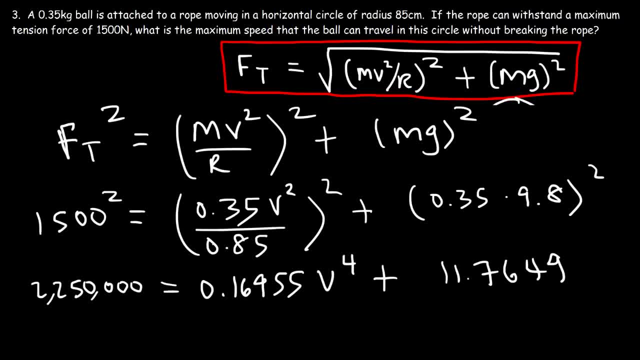 it's 11.7649.. Now, if you take this big number and subtract it by that small number, it's going to be insignificant, But we'll do it anyway. So let's subtract both sides by 11.7649.. 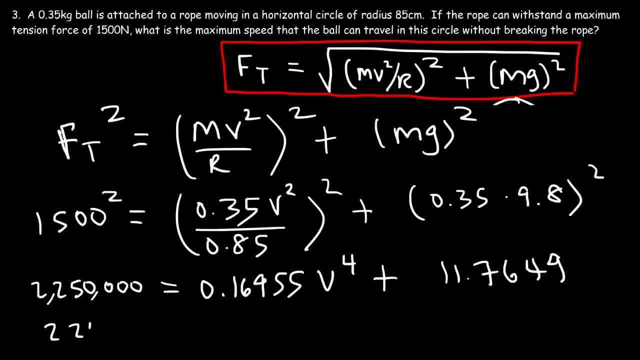 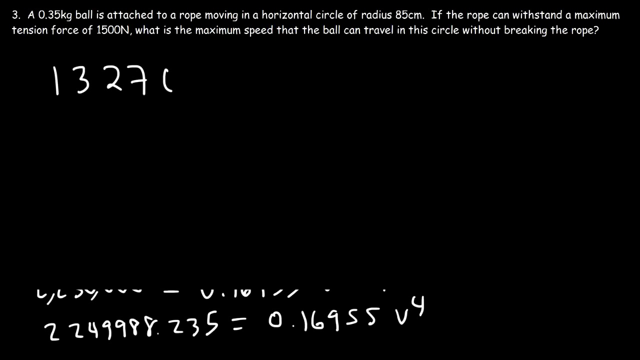 So this is going to be about 2,249,988.235.. So now let's divide both sides by 0.16955.. So you should have 1,327,035,2.32 is equal to V. to the fourth. 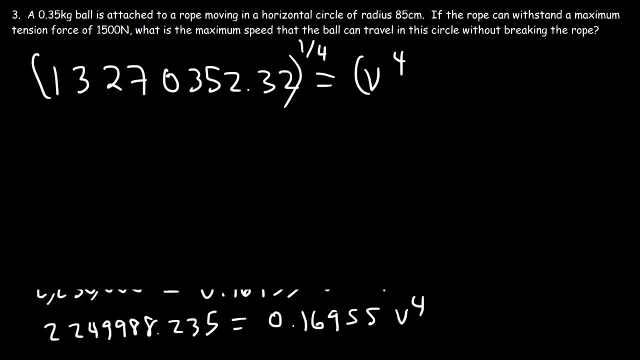 So now I'm going to raise both sides to the one-fourth power to get V. So take the fourth root of both sides and this will give you 60.356, which rounds to 60.356.. So that's going to be 1,327,035,2.32.. So now I'm going to raise both sides to the one-fourth power to get V. 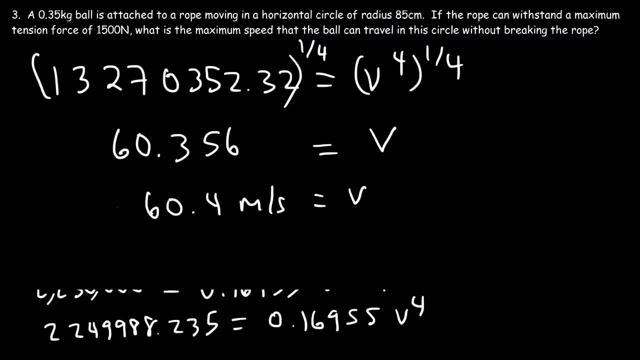 So this is going to be 1,327,035,2.32.. So now I'm going to raise both sides to the one-fourth power to get V. So, as you can see, the answer doesn't change much If the ball is moving pretty fast and if the mass is small. 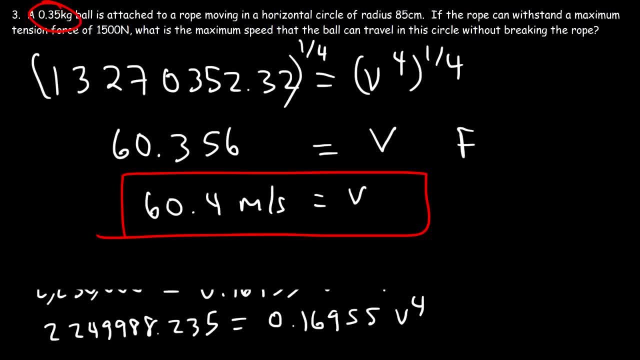 then we could say that the tension force is approximately equal to the centripetal force. So it's going to be MV squared over R if it's a horizontal circle. So if you have an object that looks like this, if it's moving in a horizontal circle, 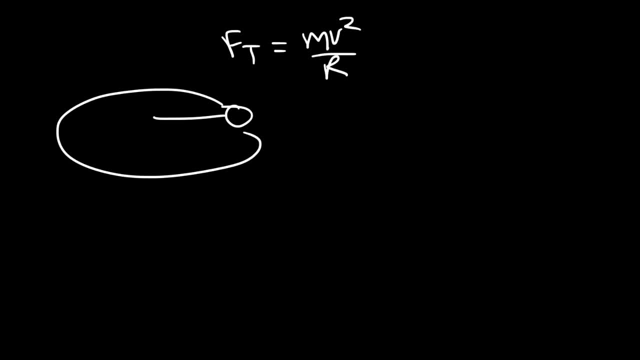 then the tension force is going to be V squared over R. force is just MV squared over R. if it's moving fast enough, If it's not, if it's at an angle, then it's different. Then you need to use this equation: It's going to be the square root of MV squared. 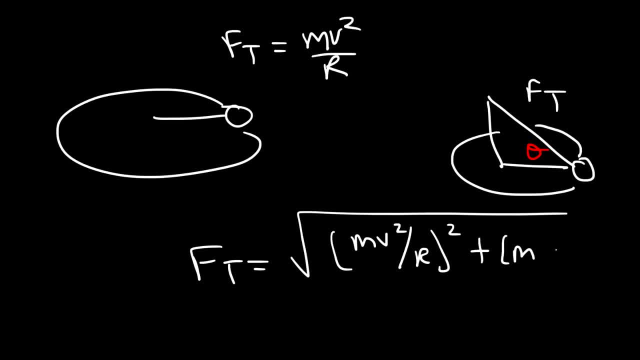 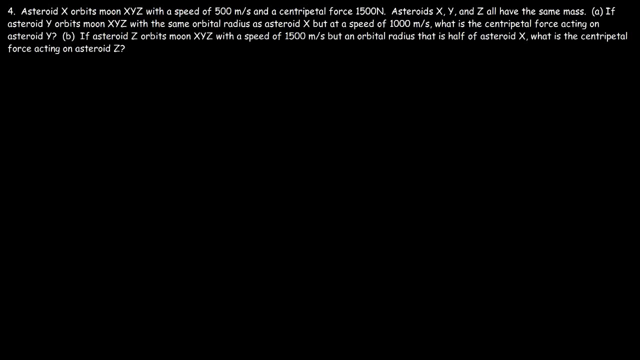 over R squared plus MG squared if it's at an angle. But that will give you the exact answer. It's just a lot more work. Here's the last problem. Asteroid X orbits moon XYZ with a speed of 500 meters per second and a centripetal force of 1,500. 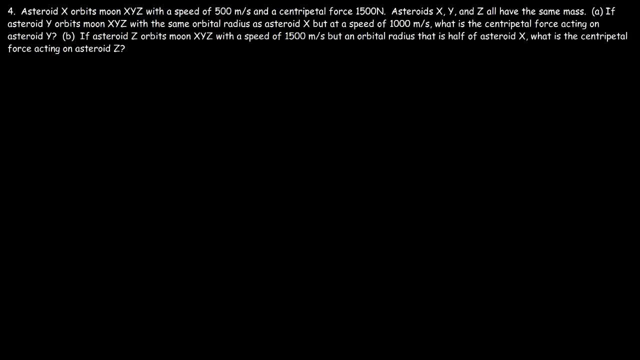 Newtons And asteroids X, Y and Z all have the same mass. Now, if asteroid Y orbits the same moon with the same orbital radius as asteroid X, but at a speed of 1,000 meters per second, what is the centripetal force acting on asteroid Y? So let's say this is a moon. 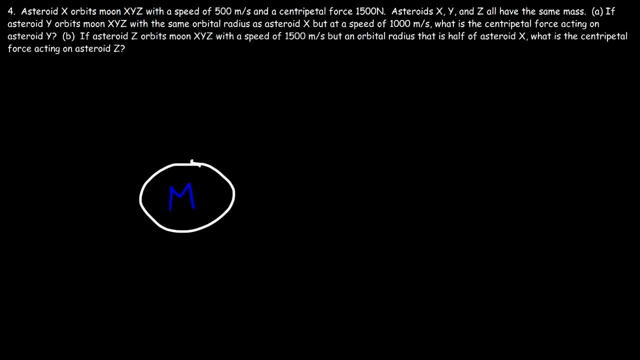 A moon that's orbiting some planet And then we have an asteroid orbiting that moon. So this is asteroid X. Now asteroid Y is in the same orbital radius as X Now. X is moving at 500 meters per second currently and asteroid Y is moving at. 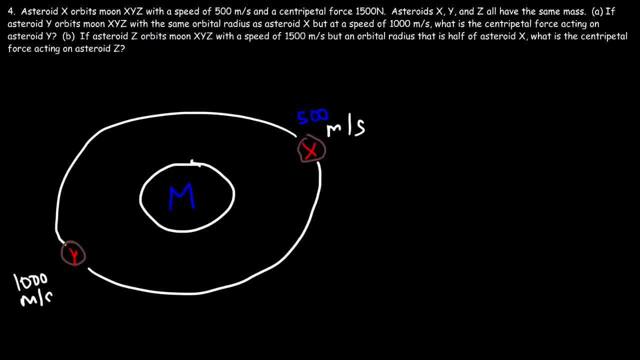 twice the speed: 1,000 meters per second. Now let's go ahead and put asteroid Z in part B. Asteroid Z is that half of the orbital radius relative to X. So somewhere here we're going to have asteroid Z, And it's going at 1,500 meters per second. Now the centripetal force on X is 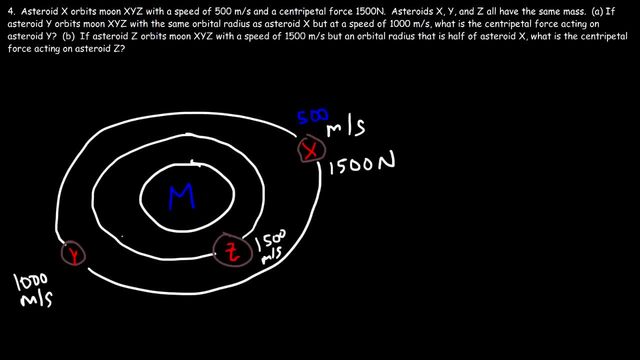 1,500 newtons. What is the centripetal force acting on Y? How can we find the answer? Well, we can't use this equation directly, We have to use it indirectly. Now, if we focus on X and Y, everything is the same. They have the same mass and the 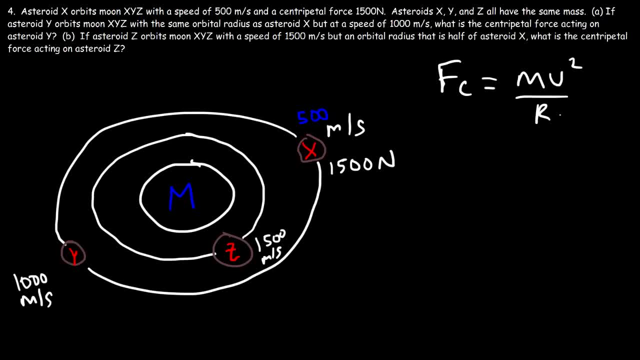 same orbital radius. The only thing that's different is the speed. Now what happens to the centripetal force if the speed is doubled? So the mass doesn't change. let's put a 1. The speed doubles and the radius doesn't change. 2 squared. 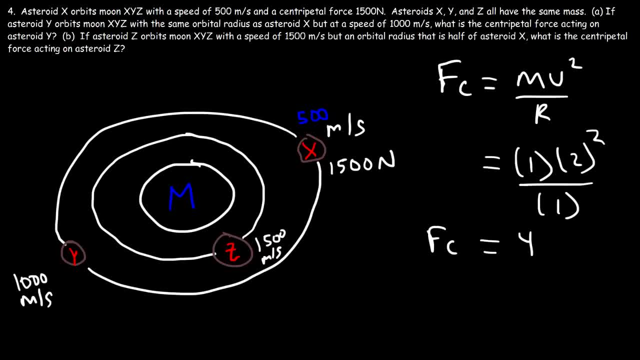 is 4.. So the centripetal force will increase by a factor of 4 if we double the speed. So if X has a centripetal force of 1,500, then Y is going to be 1,500 times 4.. 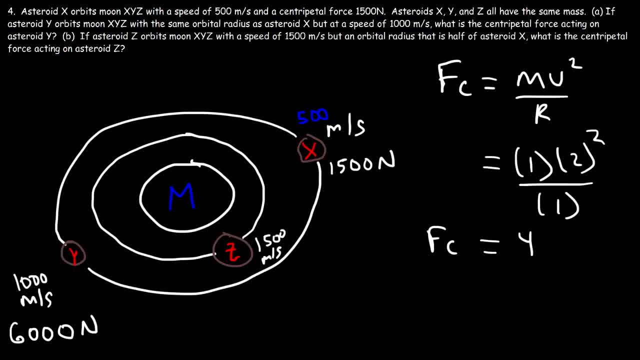 So the centripetal force is going to be 6,000 newtons. Now, if you want to come up with an equation that relates centripetal force to speed, given that everything else stays the same, like the mass and radius, here's the formula that: 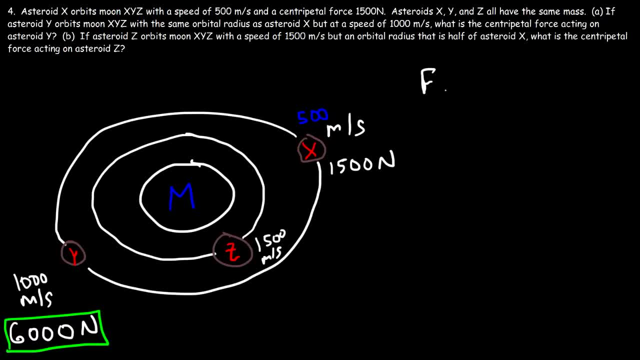 you could use. So we're going to say F2 over F1, where these two represents the centripetal force of two different objects. that's going to be M V2 squared over R divided by M V1 squared over R. Now I didn't use any subscripts for M and R because 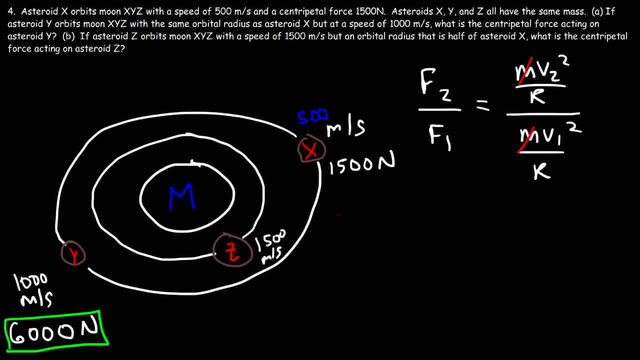 they're the same, so therefore they're going to cancel. So F2 over F1 is equal to V2 squared over V1 squared. This is the formula that you want to use. Now, if you want to solve for F2, multiply both sides by F1.. So F2 is going to be F1. 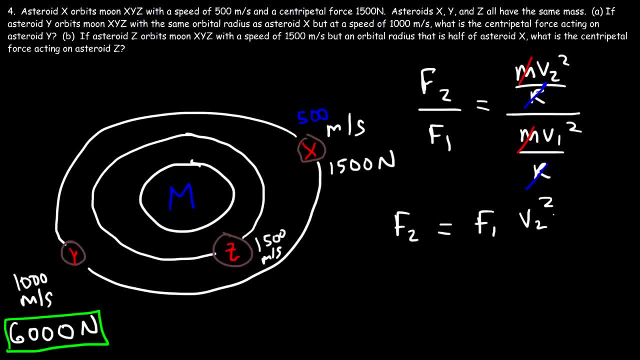 times V2 squared over V1 squared. Or you could just write it like this: if you want V2 over V1 and then square it, So let's use that formula. So F1, where 1 is the first object, asteroid X is 1,500.. The speed of asteroid X is 500 and the speed 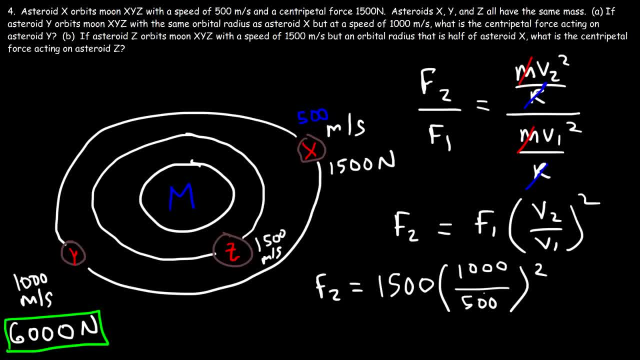 of asteroid Y is 1000.. So 1,000 divided by 500 is 2, and 2 squared is 4.. 4 times 1,500 is 6,000.. So this is the formula that you could use if you need to relate the centripetal force with the speed together. 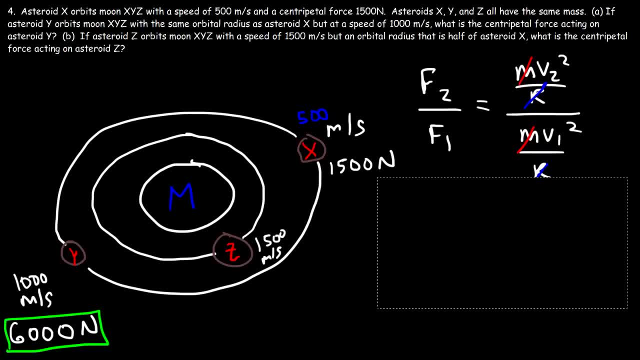 Now let's move on to the next part, Part B. if asteroid Z orbits moon XYZ with a speed of 1,500 meters per second, but an orbital radius that is half of asteroid X, what is the centripetal force acting on asteroid Z? 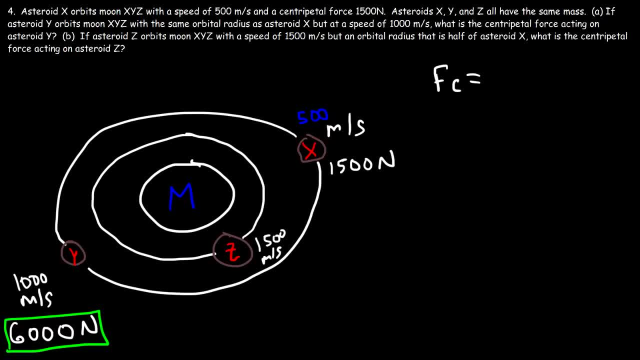 So let's think about it conceptually. The speed relative to X increases by a factor of 3. It goes from 500 to 1,500, and the radius is one half of its value. So what happens to the centripetal force if we triple the speed and cut the radius in half? 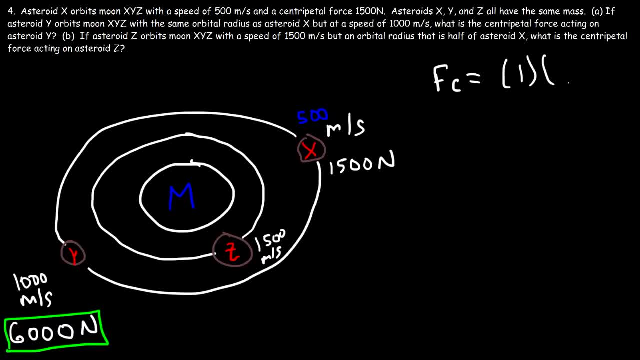 So let's use the equation. The mass doesn't change, so we're going to replace it with a 1.. The speed triples, so let's put a 3. And the radius is reduced to one half of its value. 3 squared is 9.. 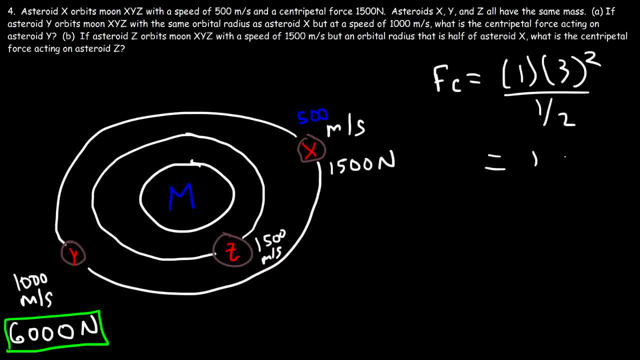 9 divided by a half, or 9 times 2,, that's 18.. So the centripetal force will be 18 times its value. So it's going to be this number: 1,500.. 1,500 times 18.. 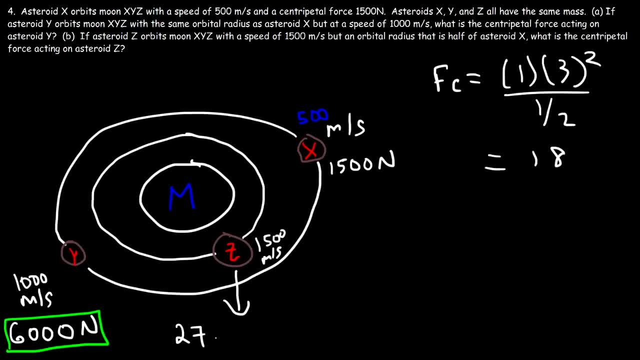 So asteroid Z is going to have a centripetal force of 27,000 newtons. Now let's confirm this answer with an equation. So I'm going to use F2 over F1 again, which is equal to M V2,. 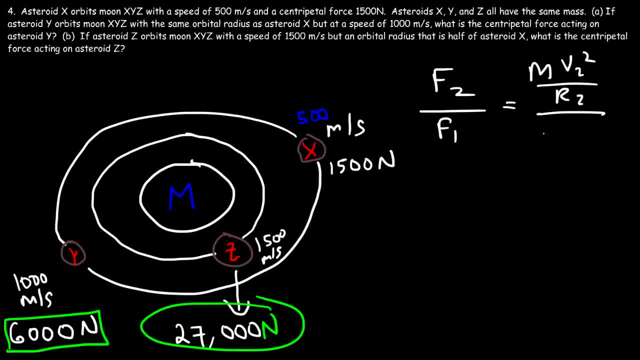 squared over R2, divided by M, V1 squared over R1.. So the only thing that's the same in this example is the mass. That's the only thing I can cancel Now using the keep-change-flip principle. if you keep this the same. 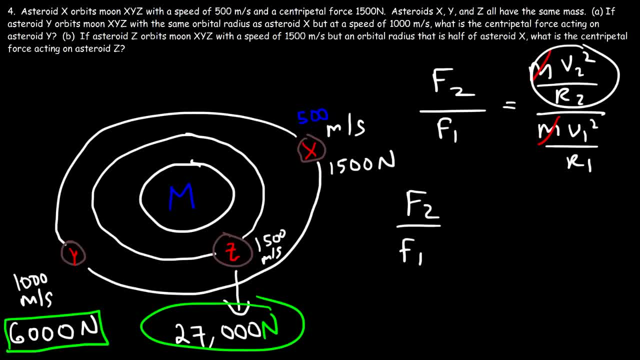 change division to multiplication and flip this fraction, you're going to get this expression: It's going to be V2 squared times R1 over V1 squared over R2.. And then let's multiply both sides by F1.. So F2 is going to be F1 times R1 over R2. 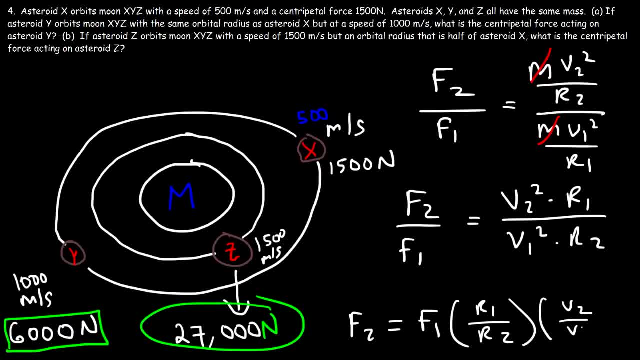 times V2 over V1 squared. So now let's plug in the values that we have. So F1, that's the original force for asteroid X, That's 1,500.. R1, we don't have a value. 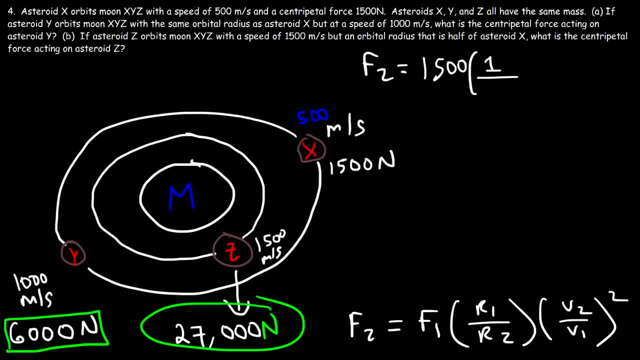 so we're just going to plug in 1.. R2 is half of R1. So it's one half. Or you could say, if R1 had a radius of 2, R2 is going to have a radius of 1.. 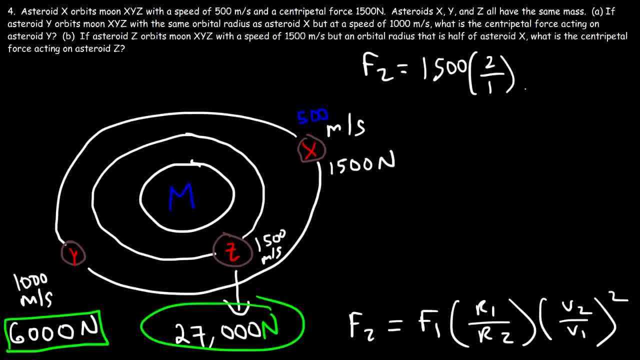 If R1 has a radius of 4, R2 is going to have a radius of 2.. Either case, the ratio of R1 to R2 is going to be 2.. V2 is 1,500.. V1 is 500. 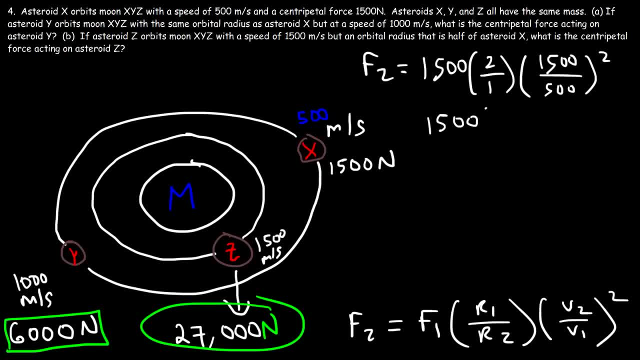 And then that's squared. So we have 1,500 times 2.. And then 1,500 over 500 is 3.. 3 squared is 9.. And 2 times 9 is 18.. So then we have 1,500 times 18.. 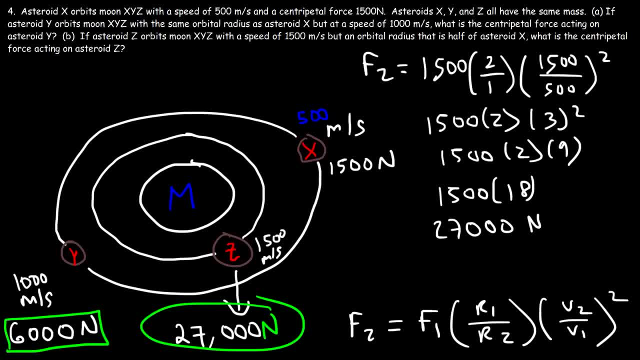 Which is going to be 27,000 newtons. So that's how you can get the answer. Now let's see if all of this makes sense. So asteroid X is moving slow And it's making the Y-turn. 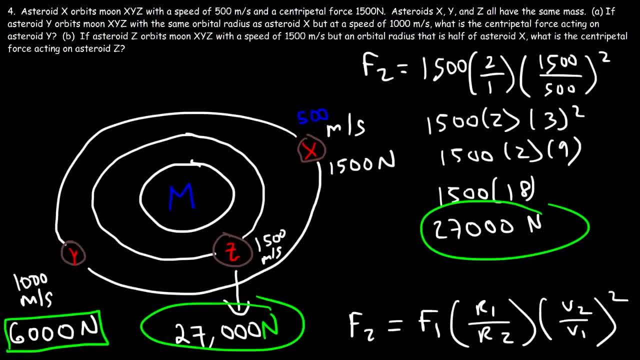 So therefore the centripetal force is very small. Asteroid Y makes the Y-turn like X, but it's moving faster, So it has a much larger centripetal force. Asteroid Z makes a sharper turn And it's moving very fast. 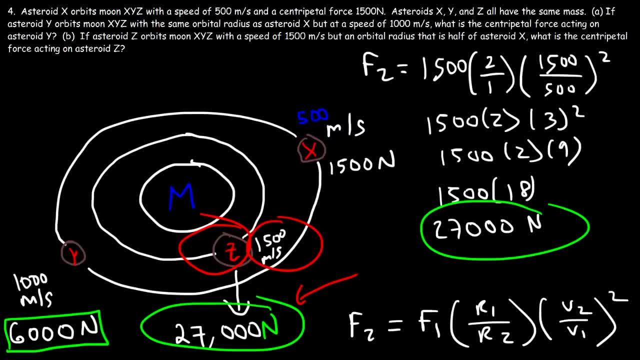 So it has an extremely high centripetal force. So make sure you understand this concept. So if you're in a car and if you make a Y-turn, driving slow, the centripetal force that you're going to feel is very, very low. 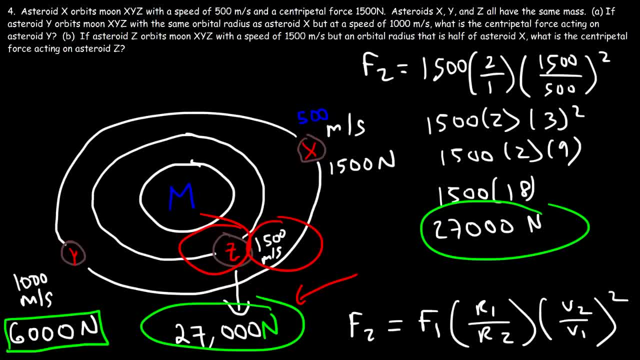 You may not even feel it at all. Now, if you make a sharp turn going very fast, you're going to feel the centripetal force. So you're going to feel the centripetal force. You're going to feel it. 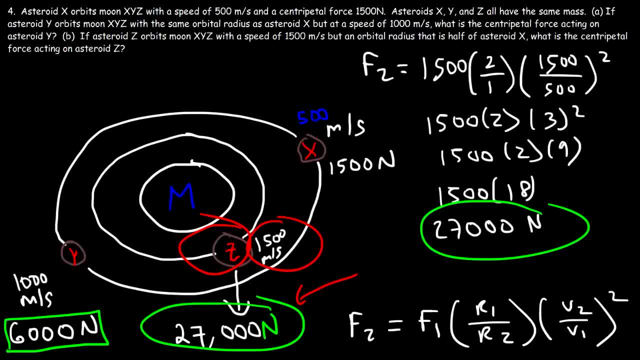 And the faster you go and the sharper the turn is, the more you're going to feel. So just make sure you understand that. And that's it for this video. Hopefully it gives you a good understanding of centripetal force. 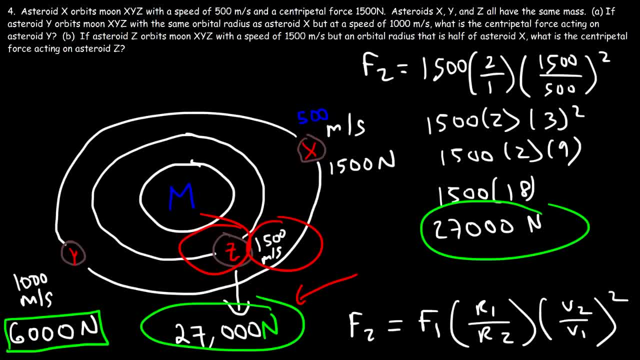 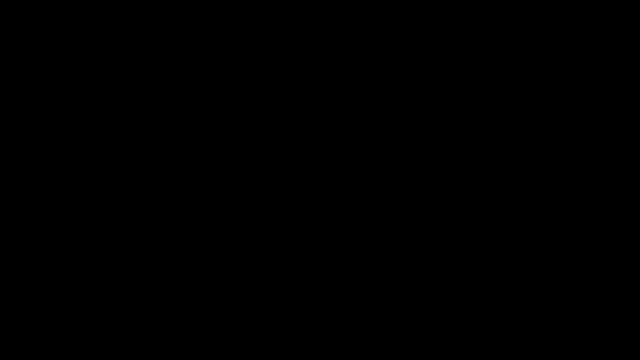 and how to solve problems associated with it. So thanks for watching. We'll see you next time.